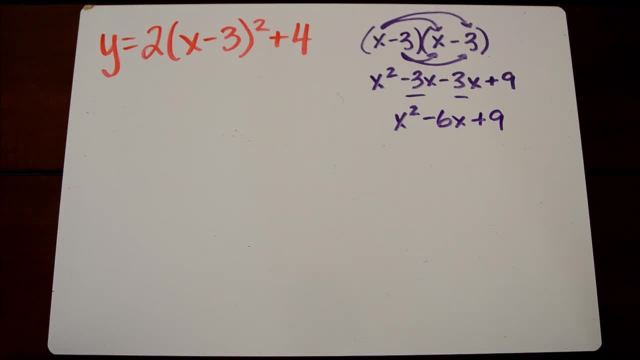 plus 9.. This isn't our answer. it's just how we start our conversion. It's going to take place of the x minus 3 squared, So let's copy everything down. but we're going to replace this where we have x minus 3 squared, And then what we're going to do is follow order of operations. We're going. 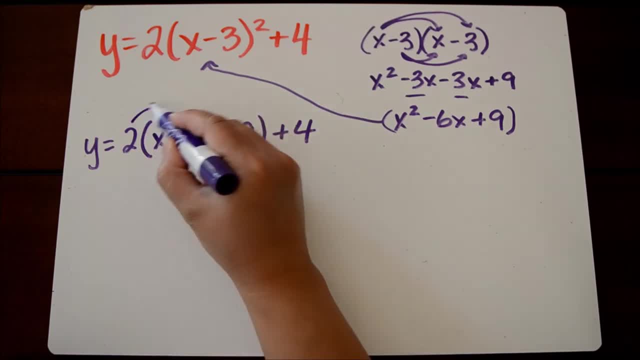 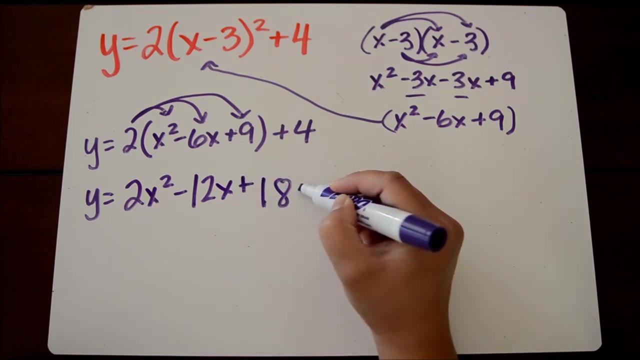 to multiply first before we add. So let's distribute the two to every term negative 3x. So we're going to get y equals 2x squared minus 12x plus 18 plus 4.. And we still have to combine like terms. So on this example, we can combine our constants 18 and 4.. So our answer, our standard. 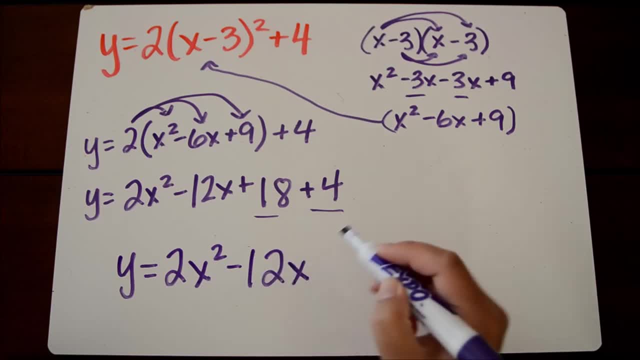 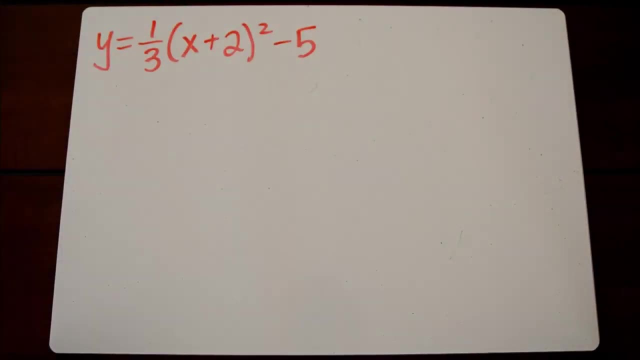 form equation is 2x squared minus 12x plus 22.. Let's take a look at one more example. This example looks a little bit more difficult because we have a fraction for our a value, But we're going to follow the same steps. We're first going to multiply that binomial x plus 2. 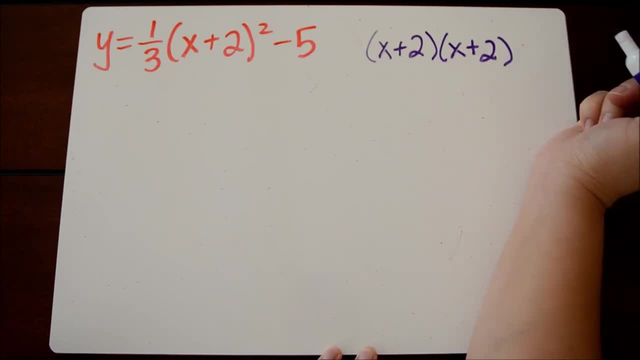 times x plus 2.. And we're just distributing every term to every term. So x times x is x squared. We're going to write: x times 2 is positive 2x, 2 times x is positive 2x And 2 times 2 is 4 combined. 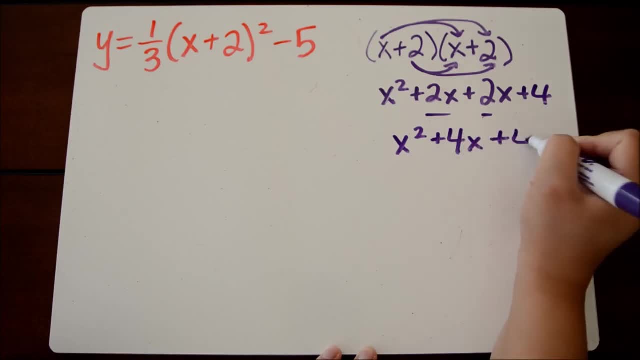 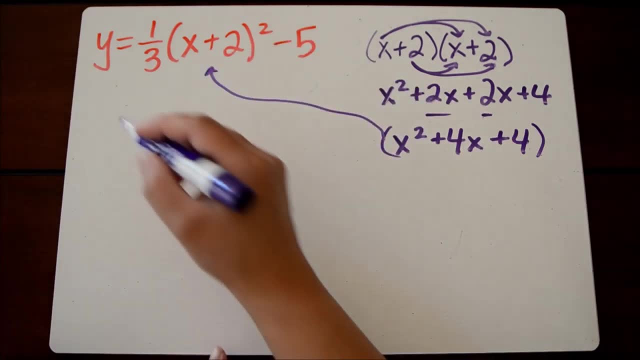 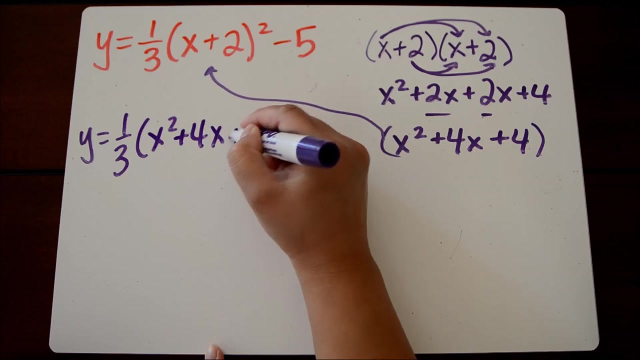 like terms. we get x squared plus 4x plus 4.. So this quantity here is going to take place of the x plus 2 squared. I'm going to copy the rest of the problem down And then here we'll write our expression that we had just multiplied with those binomials. 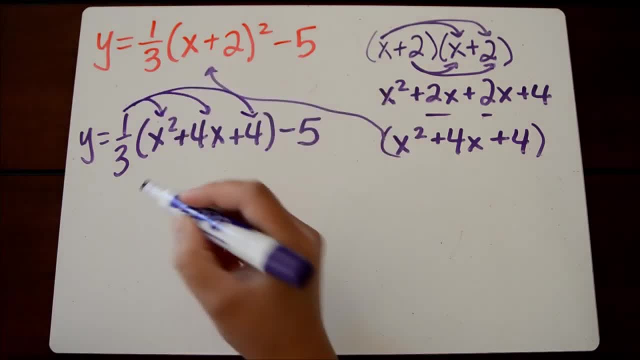 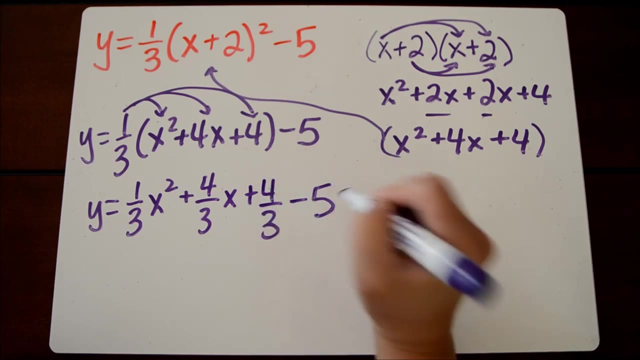 It gets a little bit tricky here because we have to multiply a fraction throughout our trinomial. So we're going to get y equals one-third x squared plus four-thirds x plus four-thirds. Don't forget, we have this minus five on the outside.